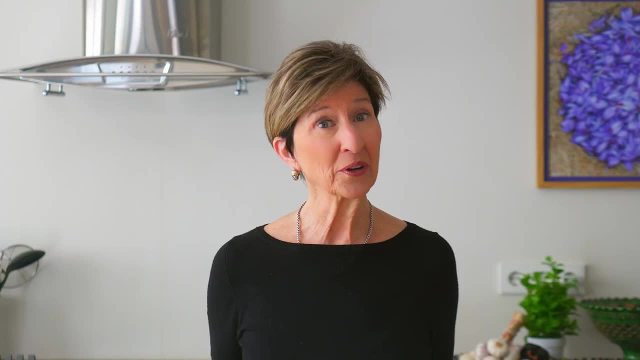 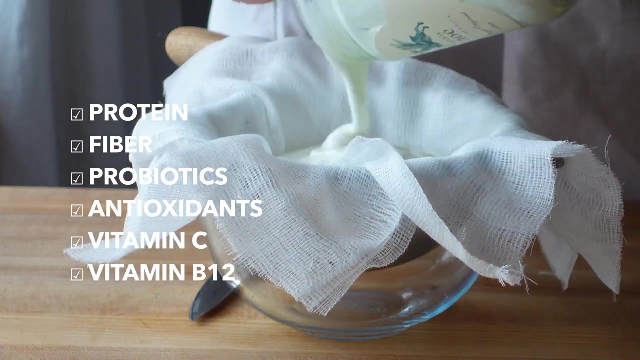 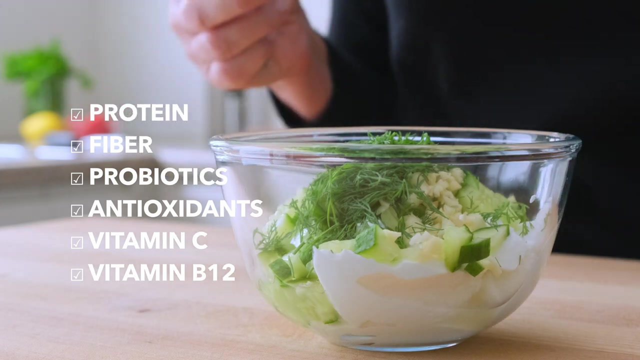 And I like to enjoy it a couple of different ways. It's super easy to let this probiotic powerhouse drain overnight and make a creamy, soft cheese, known in the Mediterranean as labne, to enjoy with whole grain crackers, Or whip up a batch of tzatziki, a really refreshing combination of Greek yogurt, cucumbers, garlic and a little. 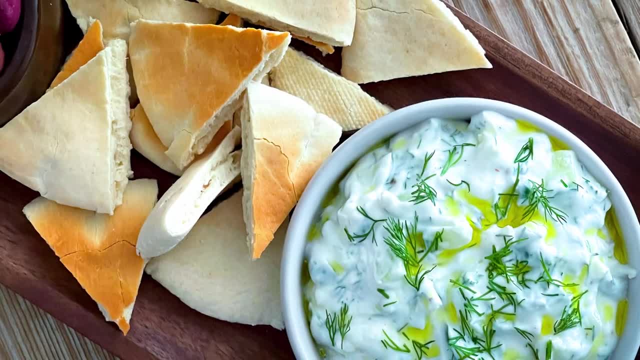 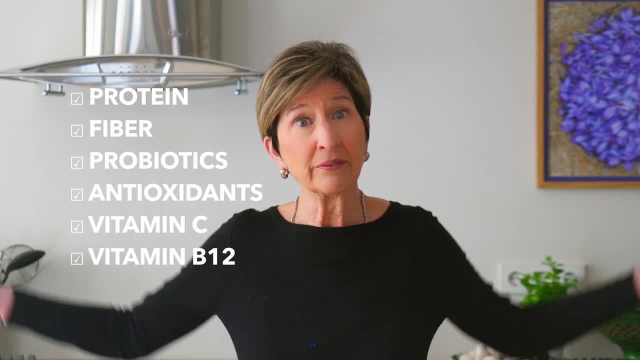 bit of lemon juice And some whole grain pita chips for dipping. It's a snack that's high in protein, fiber, probiotics, antioxidants, vitamin C, B12.. What's not to love about it? It's a snack that's high in protein, fiber, probiotics, antioxidants. vitamin C- B12.. What's not to love about it? It's a snack that's high in protein fiber. probiotics. vitamin C- B12.. What's not to love about it? It's a snack that's high in protein fiber. 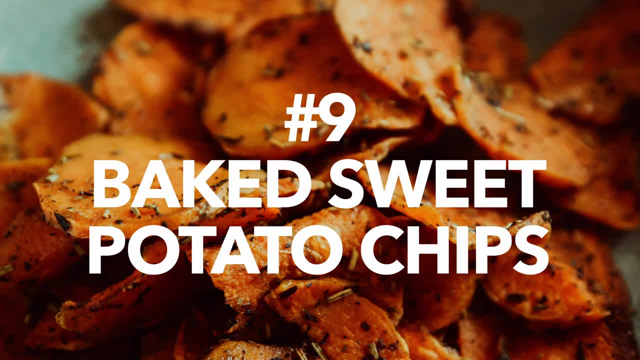 probiotics, vitamin C, B12.. What's not to love about it? It's a snack that's high in protein, fiber, probiotics, vitamin C, B12.. Number nine: baked sweet potato chips. I'm working on perfecting an air fry sweet potato. 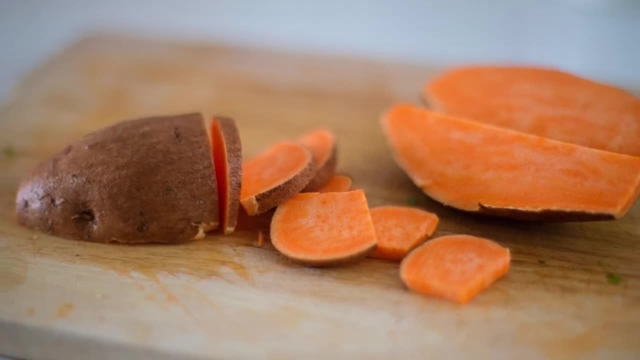 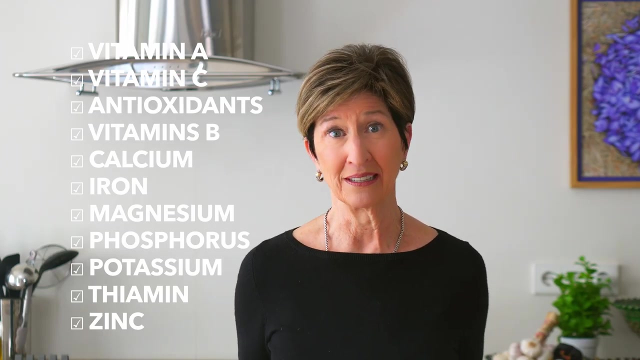 chip recipe. So I've had to repeatedly taste test these roasted crunchy snacks and I can say, for a chip lover like me, these are a pretty perfect way to get my chip fix in, Even without the recipe being quite ready for prime time. baked sweet potato chips have. 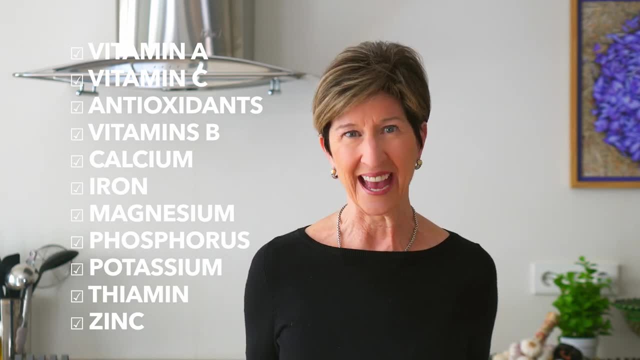 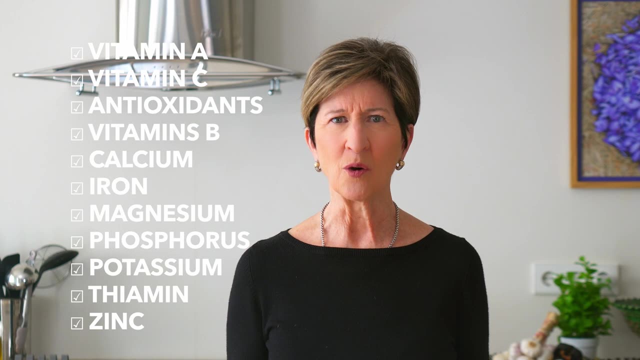 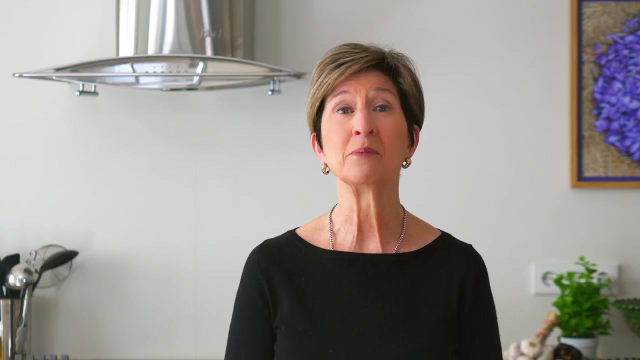 already earned a place on my shortlist for favorite snacks. Plus, sweet potatoes provide off the levels of vitamin A, and another funny fact you might not know is they can provide about half of your daily recommended amounts of vitamin C. So if you're short on oranges, sweet potato chips can. 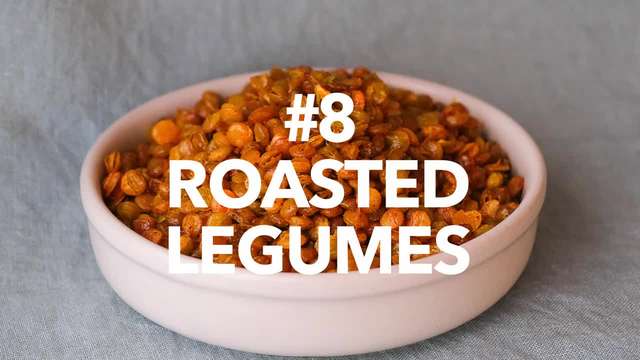 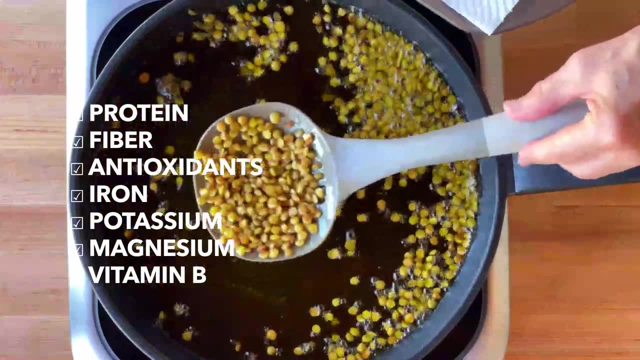 be a simple healthy swap. Number eight: roasted legumes, chickpeas and lentils. Roasted chickpeas and quick-fried lentils are perfect little snacks that are high in protein and fiber. I'll grab an occasional handful when I'm just in the mood for a bite of a little something crunchy. 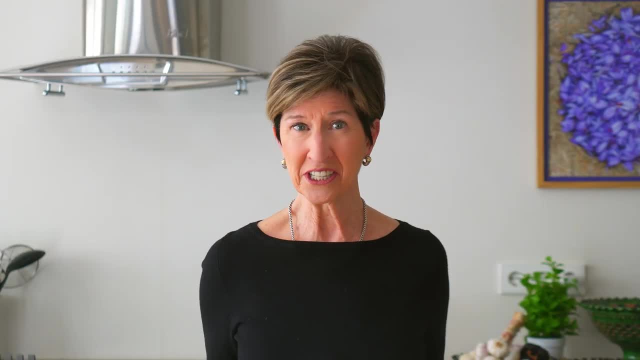 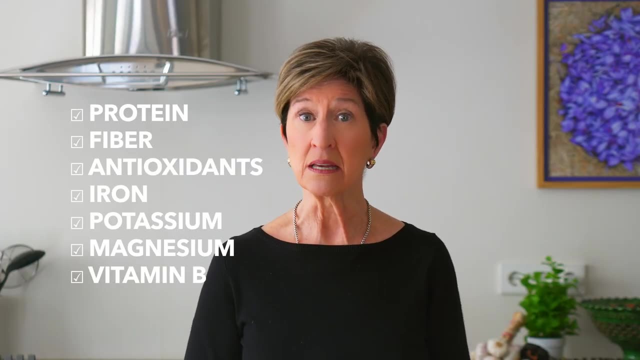 I'll toss them on a salad for an extra punch of crunch, and they're a really good source of vitamins and minerals such as iron, magnesium, potassium and vitamin B. And one of the best things about roasting these legumes at home is that you can use whatever spices and seasonings. 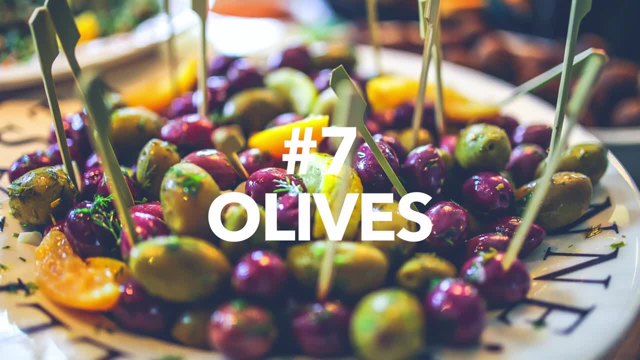 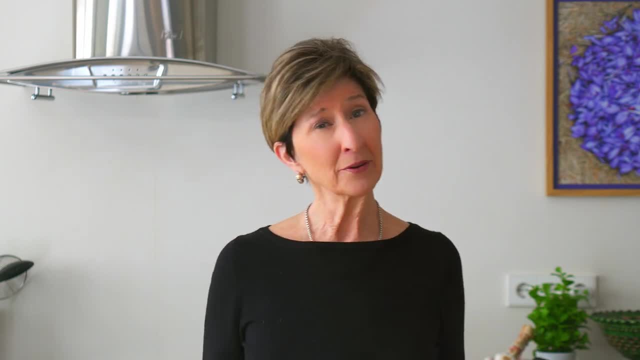 you like best and know they'll be fresh and flavorful. Number seven: olives. I've loved olives ever since George and I first started growing them in California, and my love affair has not dimmed one bit since moving to California. I've loved olives ever since George and I first started. 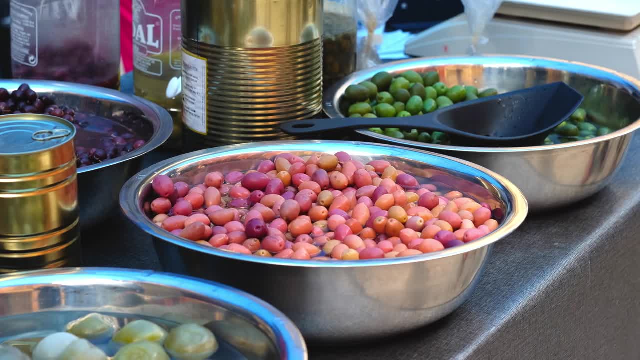 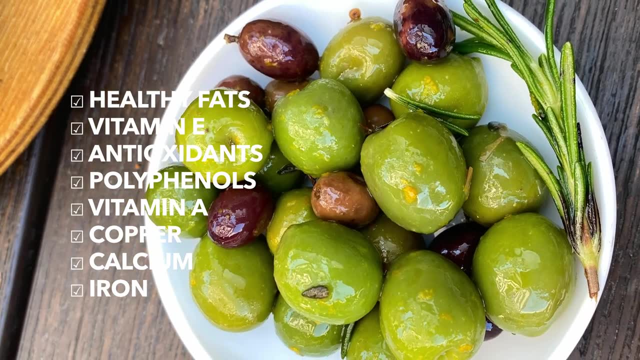 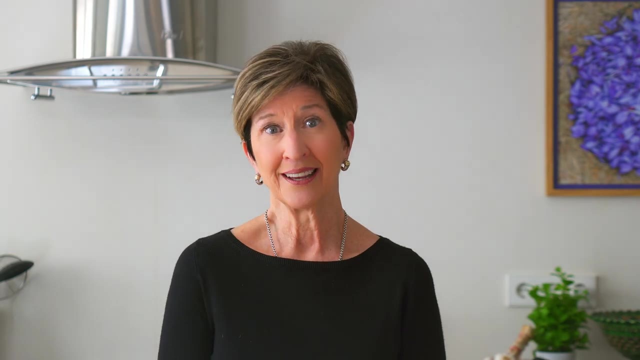 moving to Spain, where olives are the preeminent fruit, It's only been a challenge to decide which ones I like best, because this great snack option is high in heart-healthy monounsaturated fats and vitamin E, an antioxidant that helps decrease inflammation and lower blood pressure. So having 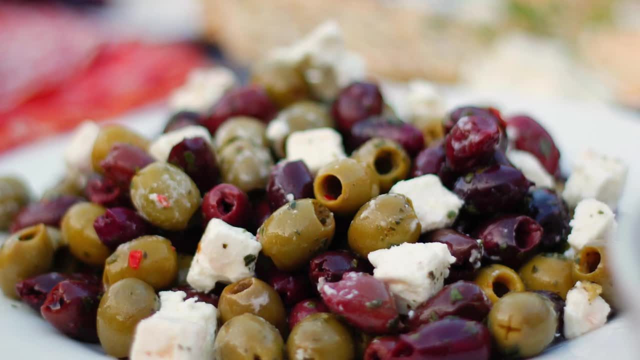 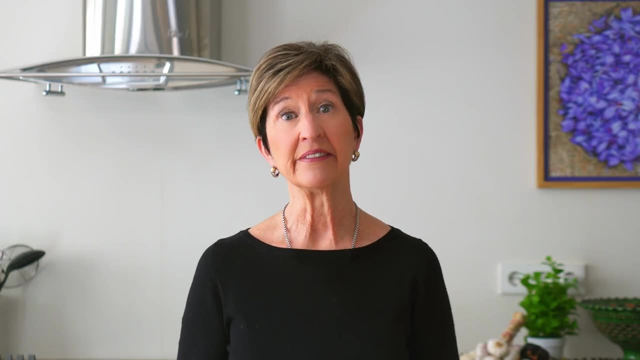 a small colorful bowl of mixed olives is a simple solution to deciding which one is my favorite. Number six: roasted nuts, Almonds, pistachios and the ultimately heart-healthy walnuts are another great snack option on the Mediterranean diet, because they're. 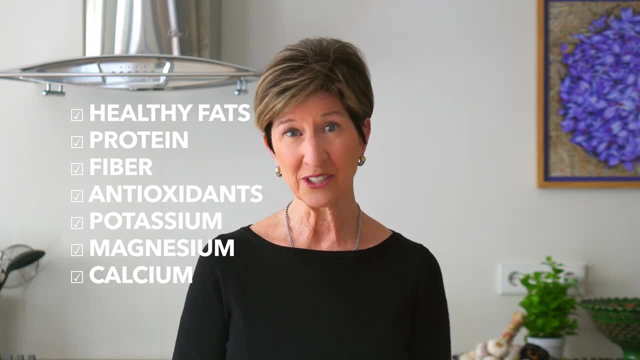 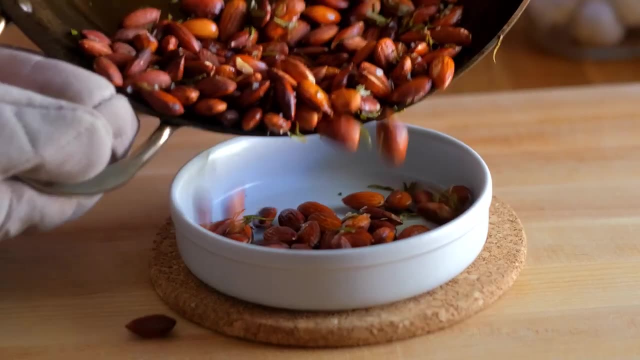 high in healthy fats, fiber and protein. They're another tasty way to stave off getting hungry. I like them most when I roast them in a pan or in the air fryer for a few minutes to bring out their nutty wonderfulness. But I have to remind myself they're pretty high in calories too. 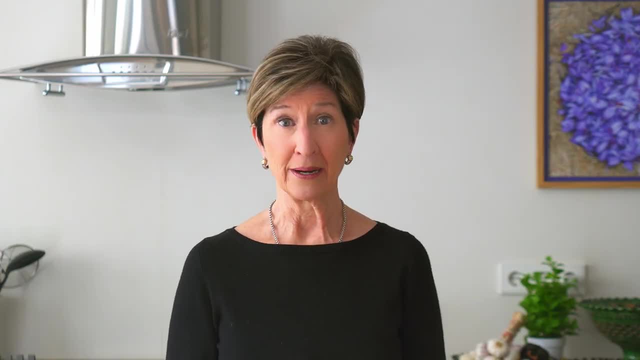 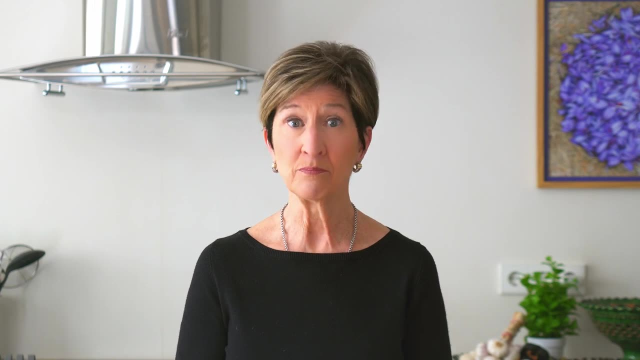 so a little goes a long way. We're at the halfway point and you can already see Mediterranean snacks aren't just mindless fillers. Each one is great at playing a small part in boosting the nutrient value in your diet. But before we continue the countdown, I have one little favor to ask: If you're a subscriber and 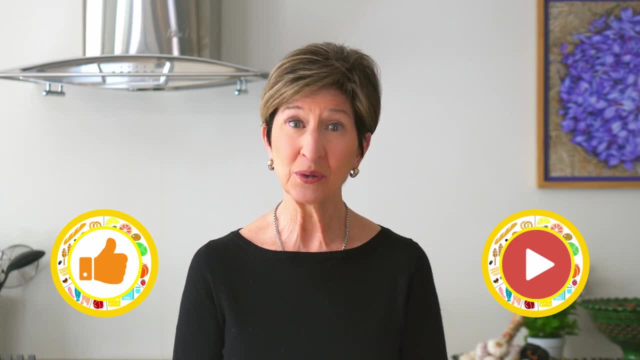 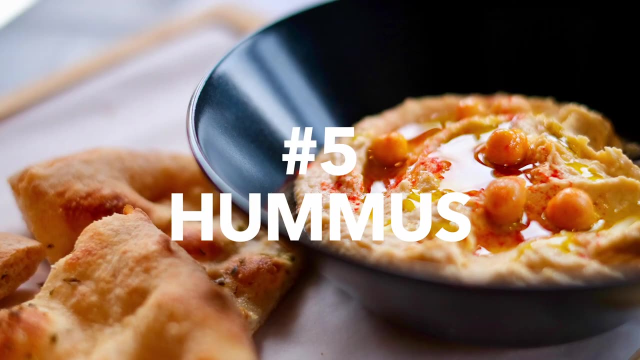 enjoying the video. please give it a thumbs up And if you're new to the channel, I'd love to extend a welcome and an invitation to join us on this healthy journey by subscribing. Now back to the countdown with number five: hummus and veggie sticks. 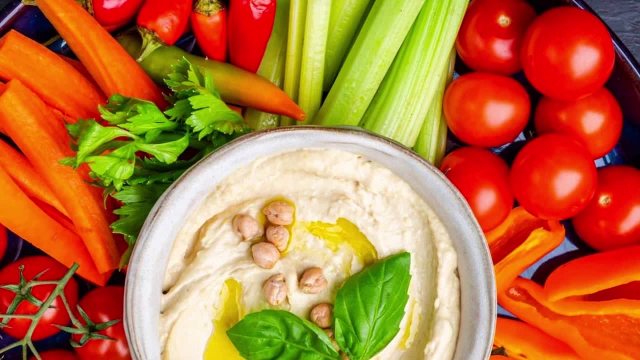 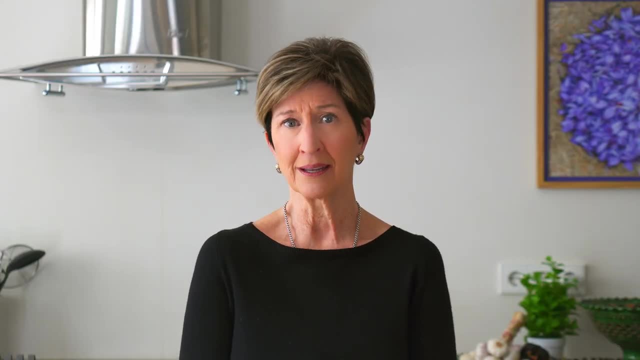 Refreshing veggie sticks with hummus is a classic snack option on the Mediterranean diet. The centerpiece, hummus, is a creamy dip made from chickpeas, tahini, lemon juice and garlic. It's an excellent source of fiber, protein and healthy fats, which can help you feeling full and 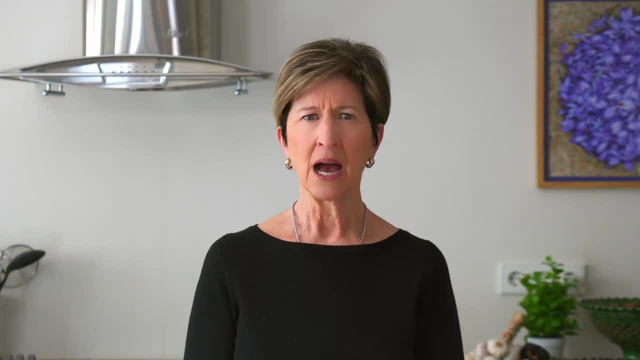 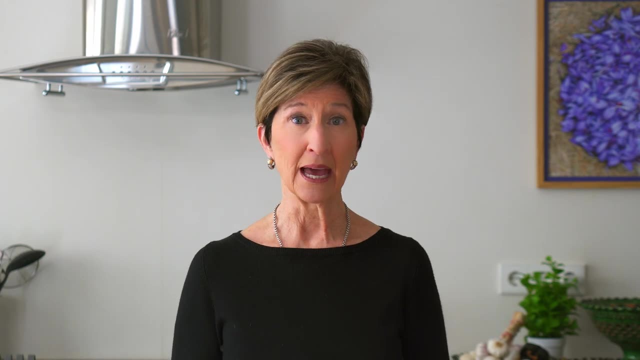 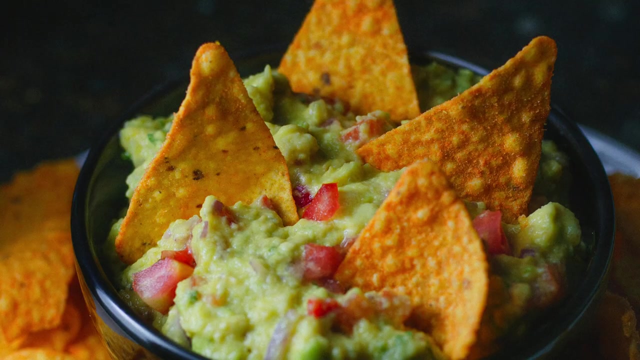 satisfied. I know if I have a little bit of tapas time I won't be very hungry for a big dinner. Number four: guacamole. A few weeks ago lots of you chimed in on a community poll about your favorite snacks and guess what Fresh fruit won the day. But I suspect that if guacamole and chips 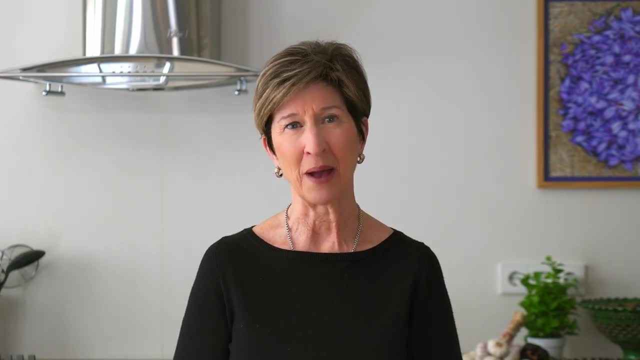 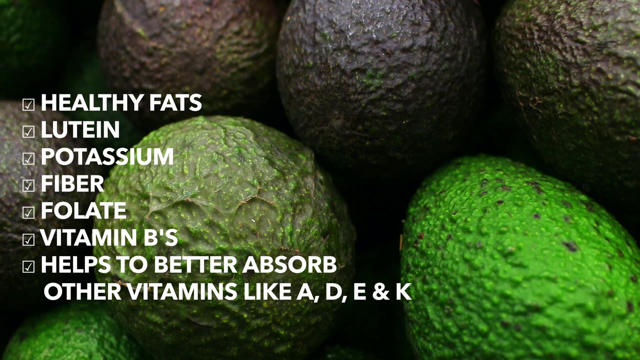 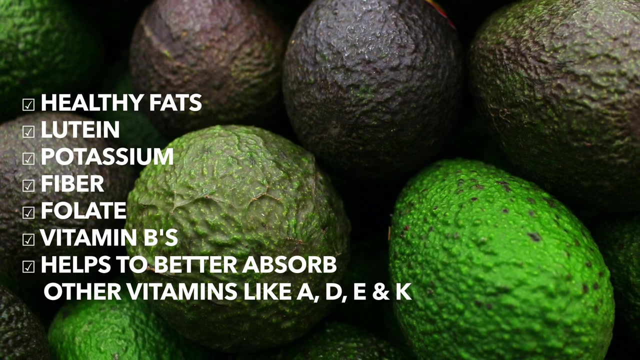 had been an option, it might have edged out fresh fruit for the top spot. The big plus of this snack? It's packed with the healthy benefits of the amazing avocado, high in heart-healthy monounsaturated fats like omega-9 fatty acids. It even helps your body better absorb vitamins like 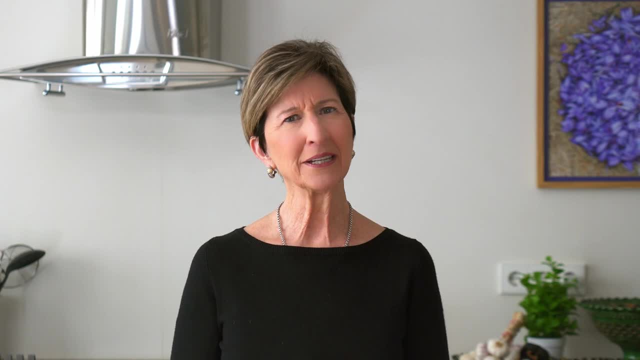 A, D, E and K. Just be aware it's pretty darn high in calories. so if you're trying to lose or maintain your weight, limit your portion to about half of a medium avocado and follow another of the Mediterranean diet guidelines. enjoy some company when you eat it and share that bowl with. 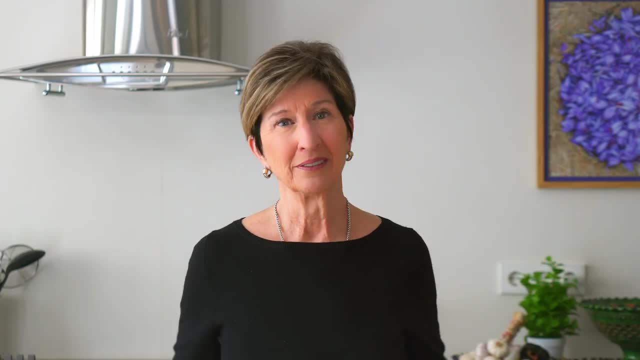 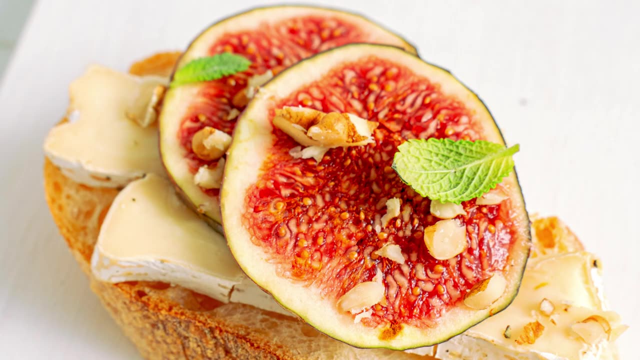 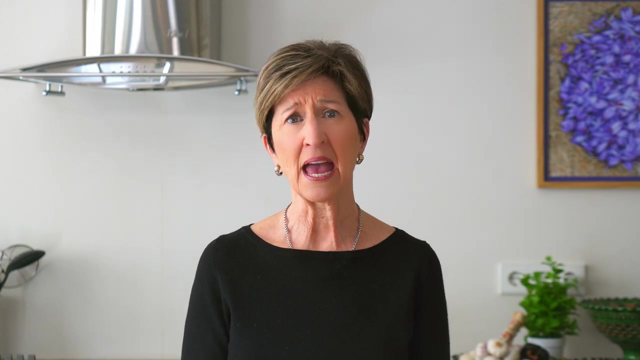 somebody else. Number three: fresh fruit. One of the fundamentals of eating the Mediterranean way every day is to pack in five fruits and veggies, and sometimes that might seem like a tall order. so what better way to add your daily count than with a simple, healthy snack of an apple or an? 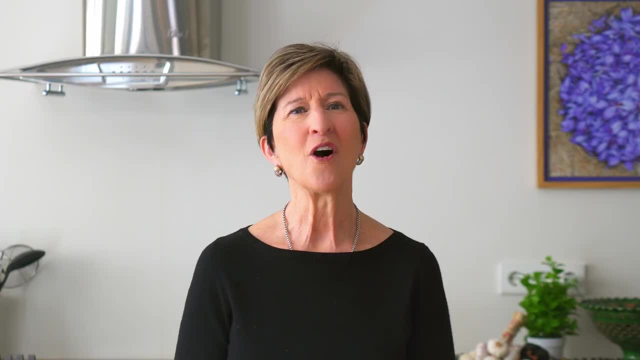 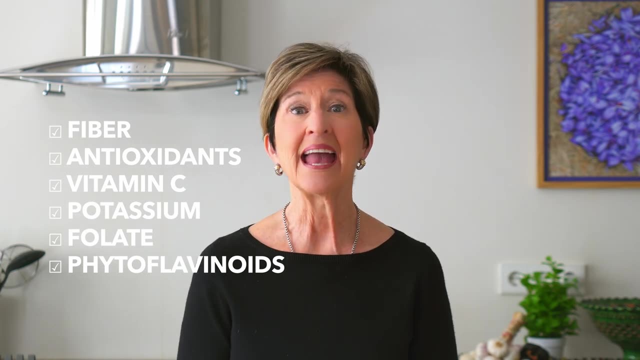 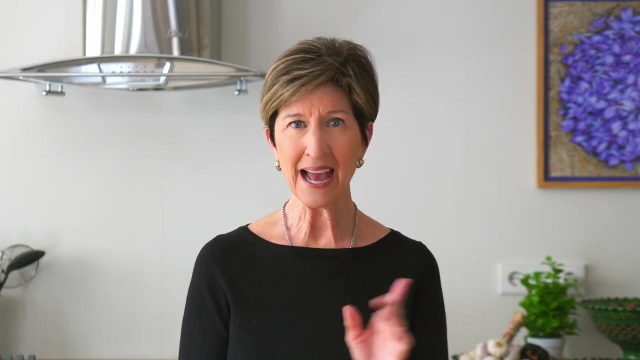 orange, or some grapes, or some seasonal berries. All these fruits are naturally high in fiber, vitamins and minerals, including vitamin C, potassium and folate. And eating fresh food is so much better than grabbing a candy bar or a sugary drink to satisfy your sweet tooth Once you get onto it. 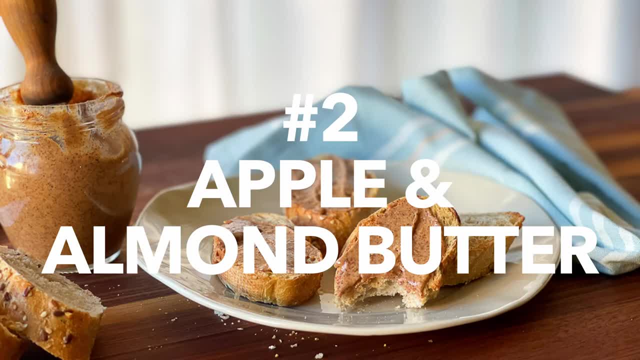 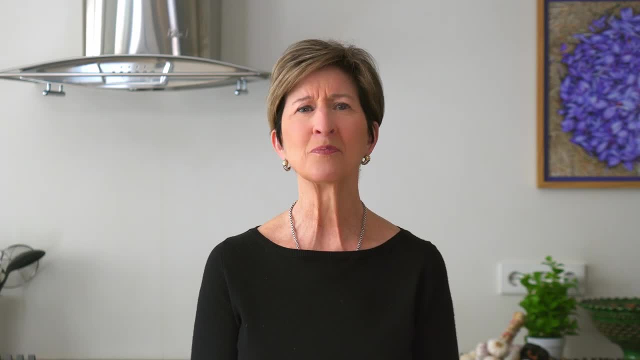 you'll find it's one of the best snack options in your arsenal. Number two: apple and almond butter. A simple slice of apple smeared with a touch of homemade almond butter is my idea of the perfect snack. I make almond butter almost every week from our own homegrown almonds. Nothing could be simpler. 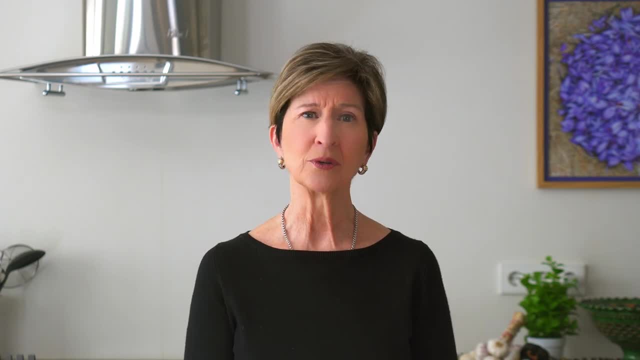 and handier to have on hand when we enjoy it as a snack with some slices of crispy crunchy apple. And finally, my favorite snack of all time, number one, dark chocolate. Maybe chocoholic is too strong a word to describe me, but all my life I've enjoyed this Mediterranean favorite. 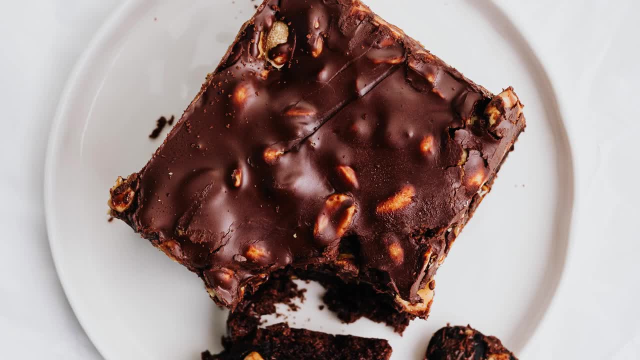 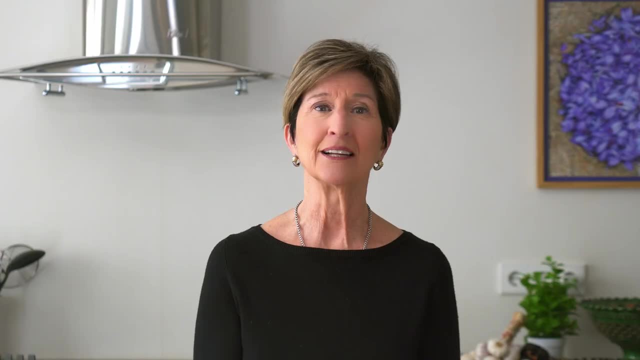 intensely rich, super dark chocolate and passed out milk chocolate every time, And it doesn't take much to satisfy my craving. Just a little bit and you're ready to go, And in exchange I gain a little boost of flavonoids, antioxidants, that. 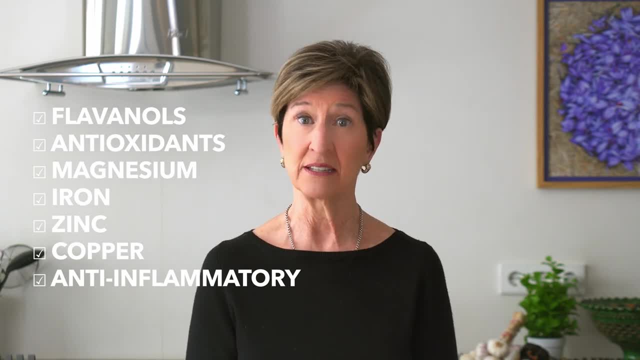 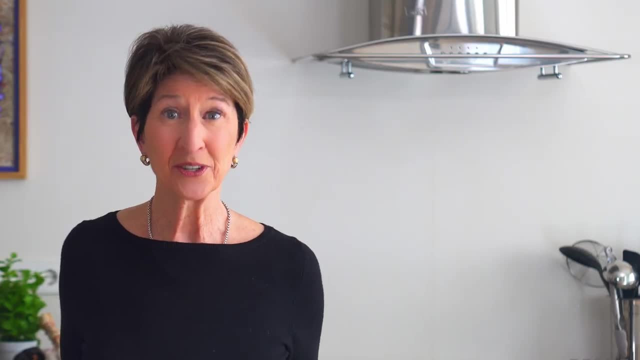 protect the body against heart disease and stroke, and all the healthy qualities of magnesium and iron, which makes me feel even better about my number one choice. Always remember: incorporating these snacks into your daily diet doesn't have to be complicated With the right ingredients. 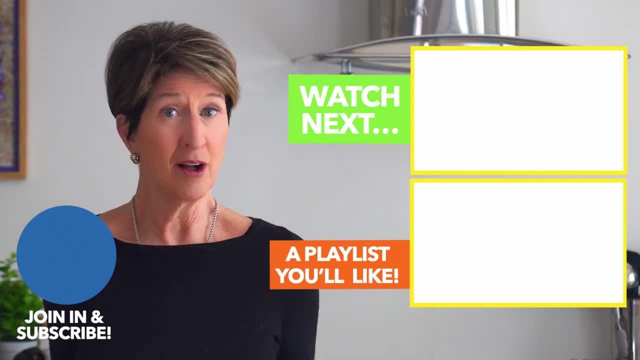 and a little creativity, you can create healthy, delicious snacks to enjoy all day long. And when you're looking for something sweet, savory or crunchy, there's plenty of options to choose from, And you can find them if you click on this playlist right now.